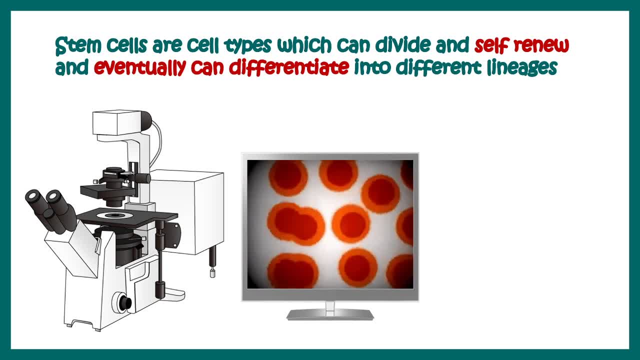 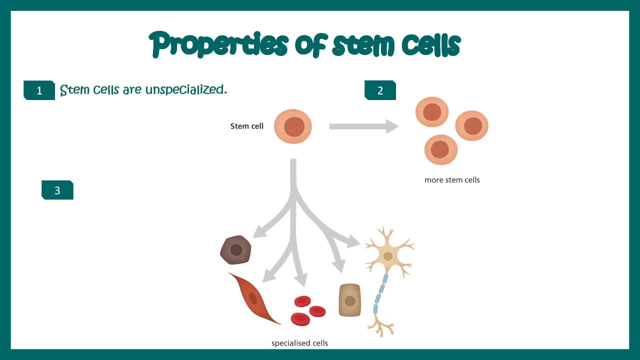 they can be differentiated into different lineages. So let us talk about the properties of the stem cell. First of all, stem cells are unspecialized. Second, stem cell have self-renewal properties. and third of all, stem cell can be differentiated into different lineages, and that is nicely depicted in this image. 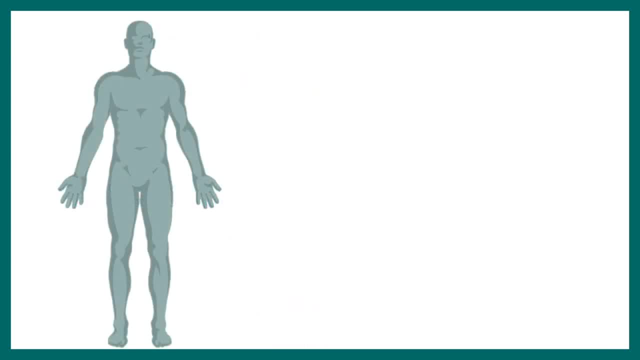 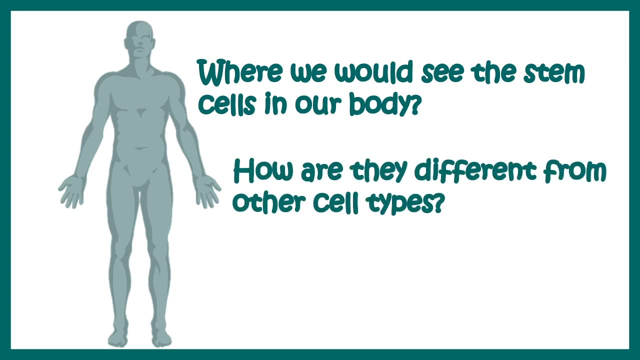 So let's talk about few important things, that where we would see the stem cells in our body. How are these stem cells different from any other cell type present in the body? What are the properties that the stem cells have in our body and what is the relevance of these stem cells? so if we look at our 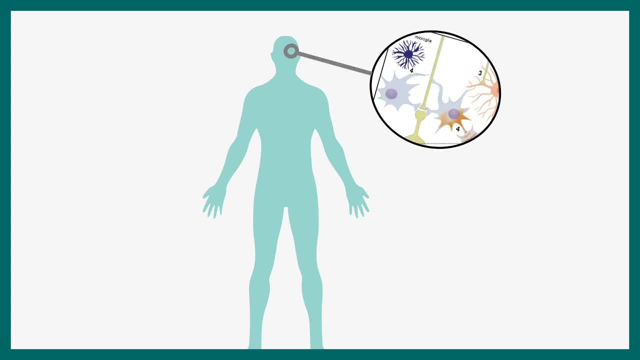 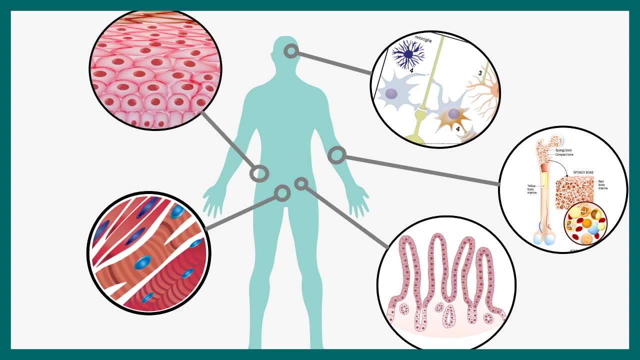 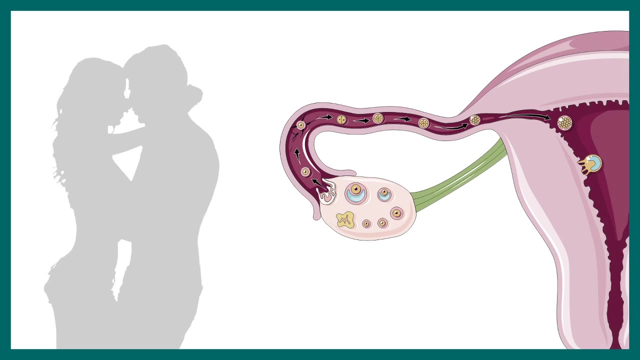 body. we would find stem cells at various locations, such as in our brain, in the bone marrow, in the intestine, in the muscles or even in the skin, so their distribution is pretty wide. now let me tell you there are different categories of stem cell. so the first stem cell that I'm going to talk about is our zygote. 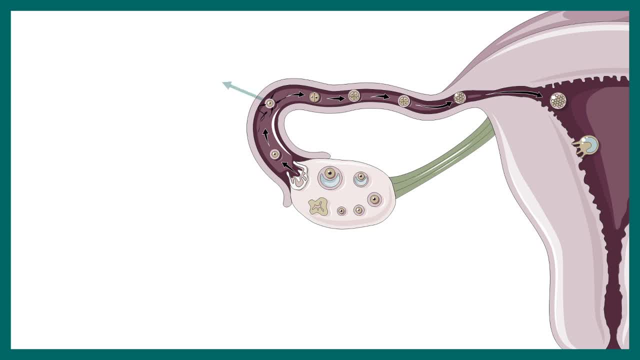 so after fertilization, you know, zygote is formed and zygote divides to two cell stage, four cell stage, eight cell stage and eventually it would get implanted into the endometrium lining. at a blastocyst stage it turns out the zygote. 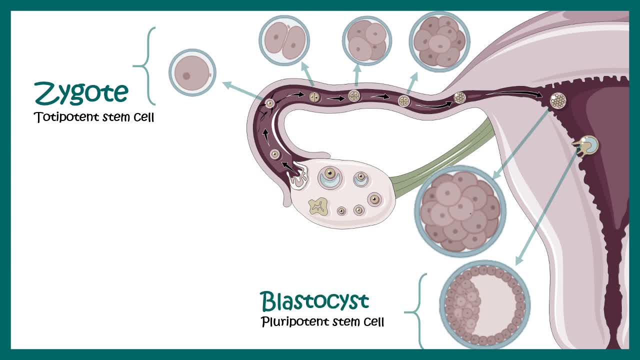 is known as a totipotent stem cell, whereas the blastocyst is known as a pluripotent stem cell, or blastocyst is the source of pluripotent stem cell. now you must be confused with the term totipotent or pluripotent, so let us analyze the term. 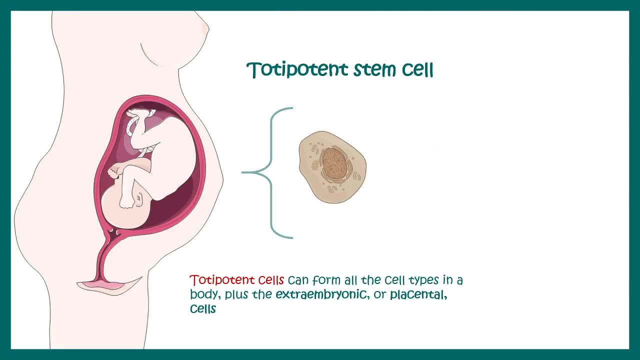 in a bit more details. totipotent stem cell means these cells are super potent and they can give rise to all the cell types present in an embryo and as well as extra embryonic tissue. so they can give rise to embryonic tissue as well as they can give rise to extra embryonic tissue. 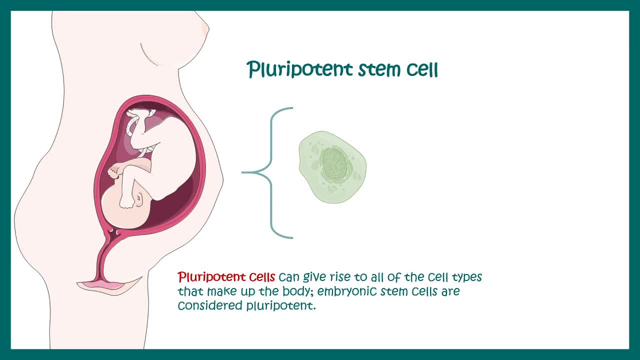 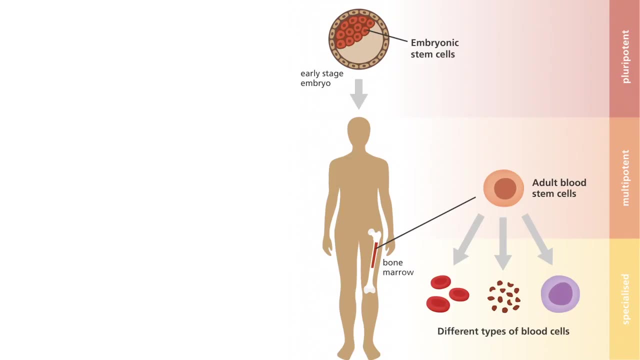 such as placenta. but a pluripotent stem cell can give rise to all cell types present in our embryo but not the extra embryonic tissue. so the placental cells cannot be derived from pluripotent stem cells. so potency has decreased in case of pluripotent stem cell. now, as we go along, there would be decrease in the. 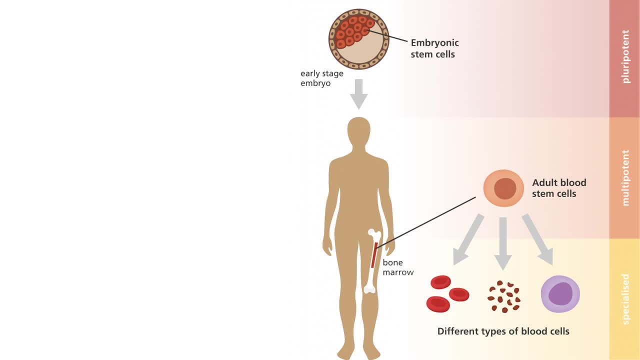 potency further decrease, such as multipotent stem cells, which can only give rise to few cell types. such as hematopoietic stem cells: they can give rise to all the blood cell type, but they can never give rise to a neuron or let's say a liver cell. so their potency is reduced and they are known as 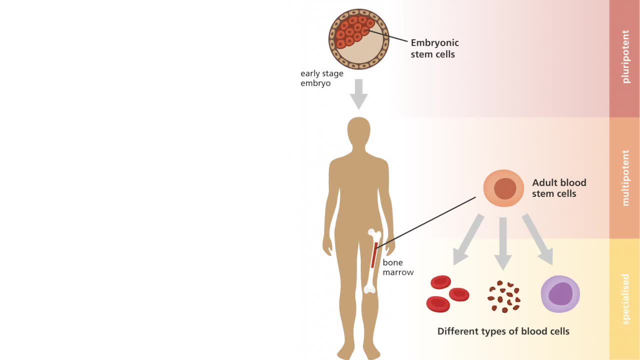 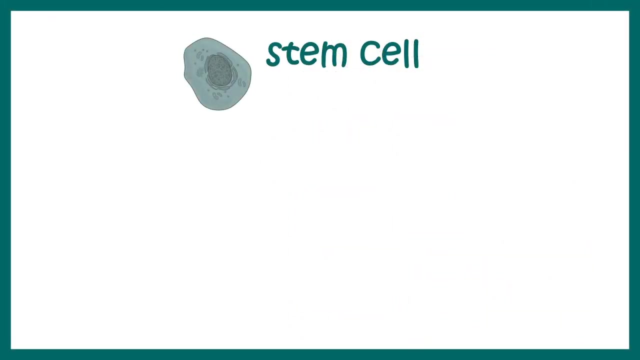 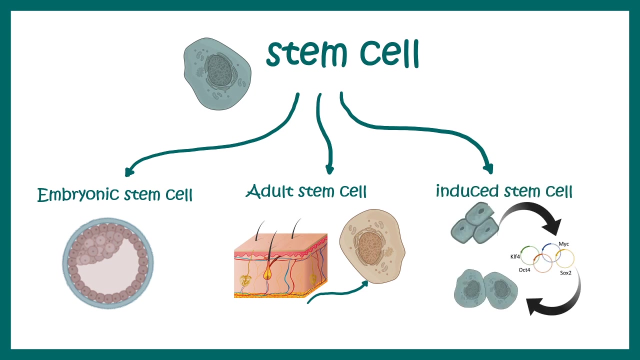 multipotent cells. now, ultimately the cells gets terminally differentiated. that means they become a particular lineage and they would never go move back to that lineage from that lineage. okay, so stem cells can be classified into three broad categories: first, embryonic stem cells, adult stem cells and induced pluripotent stem cells. so we'll talk all about that embryonic. 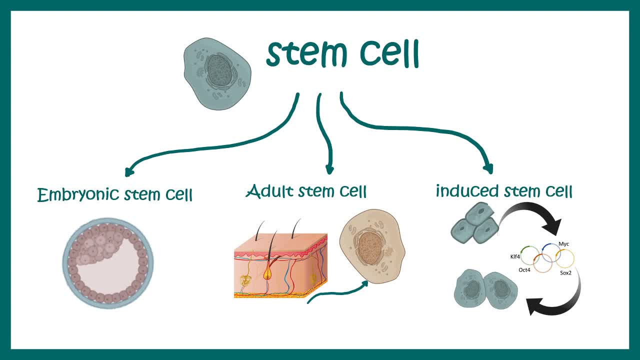 stem cell is basically derived from the blastocyst, the inner cell. mass of blastocyst adult stem cell can be found in our skin, in our hippocampus and in many places in the body. so these adult stem cells are bit more differentiated than the embryonic stem cells, but they also have some to some extent self. 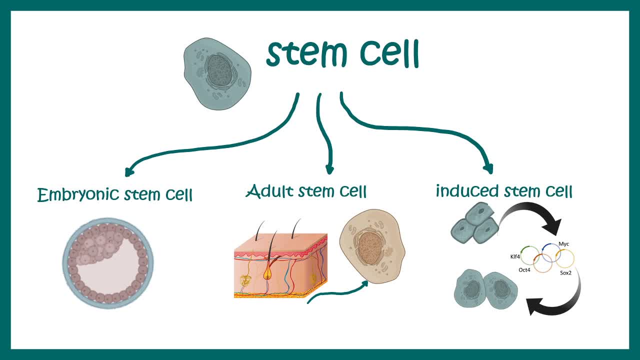 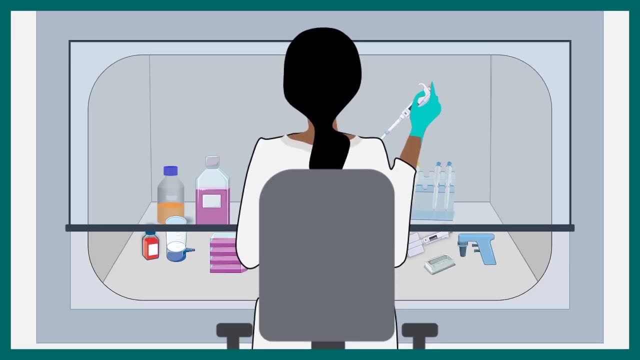 renewal property and the induced pluripotent stem cells are very interesting because any cell type that is induced pluripotent stem cell has to be type, gets converted to stem cell forcefully in this paradigm. So they are rather artificial, so they are not actually present in our body. Let us look at in the lab how stem cells are cultured. 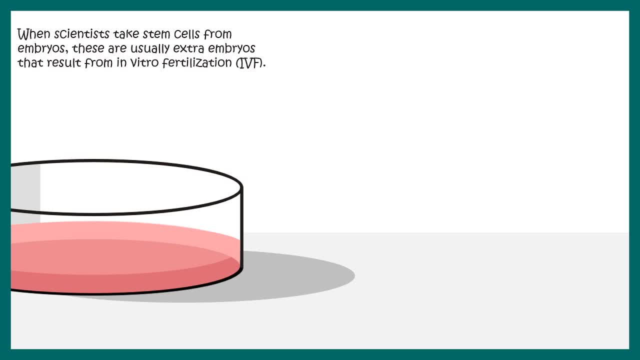 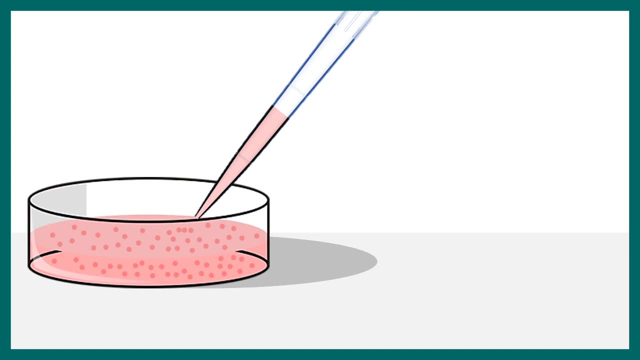 So generally in the IVF clinic there would be blastocyst from where scientists would extract the inner cell mass. After collecting the inner cell mass they would be resuspended in a cultured format. but culturing them is a bit difficult because first you need to have a bed of. 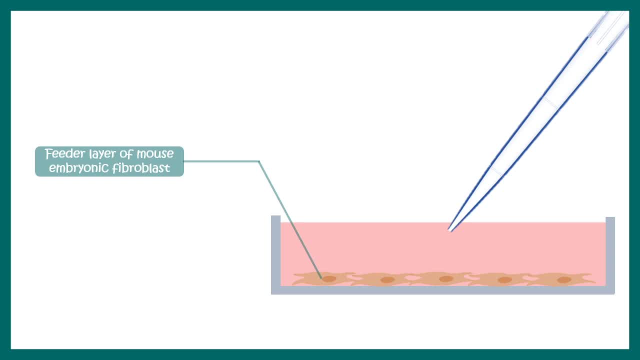 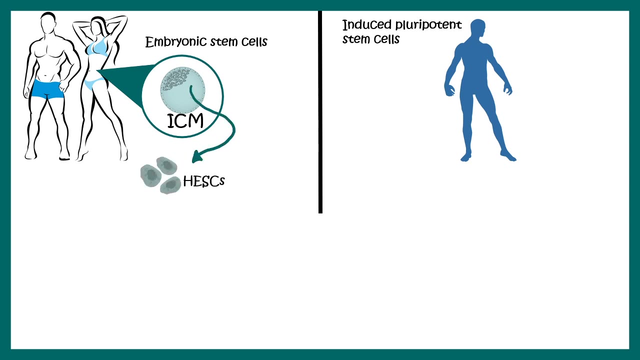 or a feeder layer of embryonic fibroblasts, and on top of that it is possible to culture these stem cells. So it's complicated to culture them Now. the embryonic stem cells can give rise to like specific cell types in our body, or it could be used to differentiate. 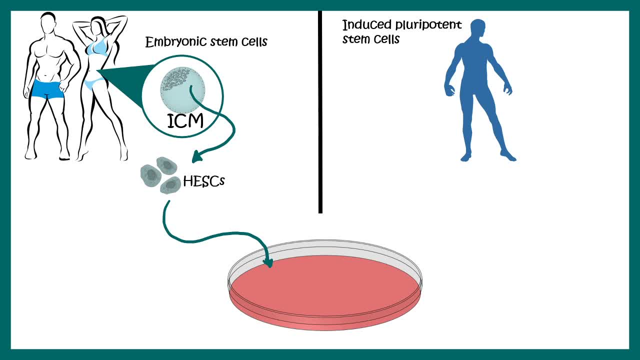 into different lilies. Now, induced pluripotent stem cell, on the other hand, is also very important because induced pluripotent stem cell can be derived from any cell type in the body, for example a skin cell. The skin cell can be transfected with specific combination of plasmids such as KLF4,. 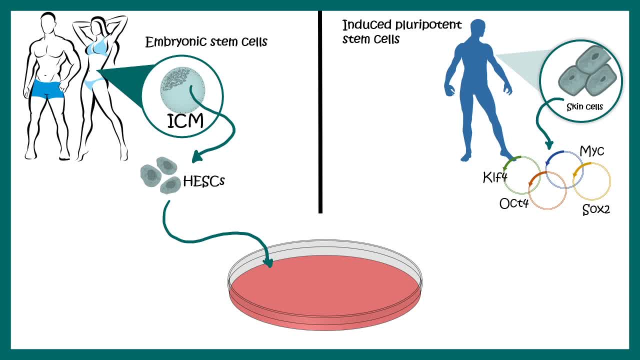 MEK, OCT4 and SOX2, which would convert these skin cells into a stem cell, or this is known as induced pluripotent stem cell, because we forcefully induce these cells to be a stem cell. Now this induced pluripotent stem cell can also be cultured and can be. 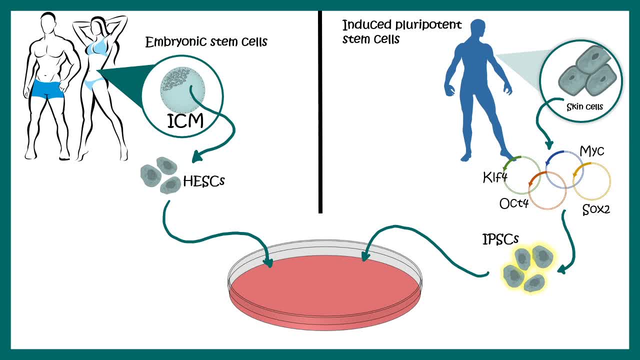 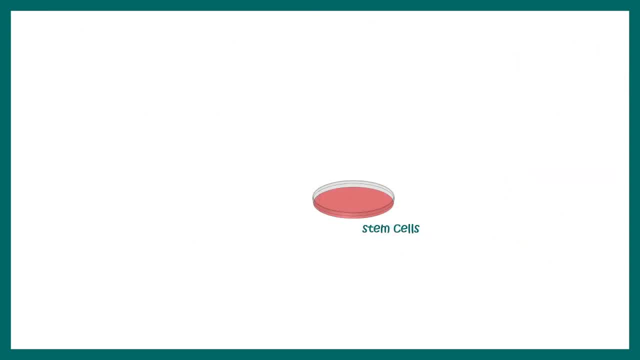 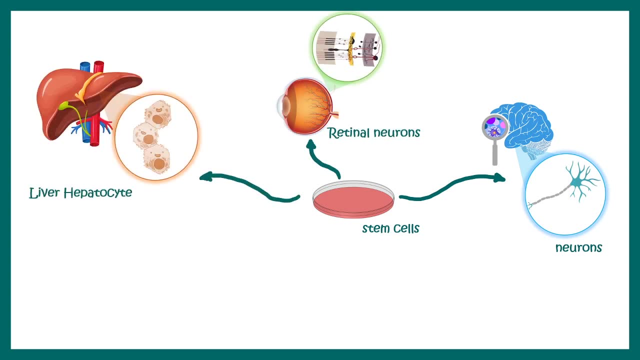 differentiated into different lineages. So these are very interesting and both of these procedures has therapeutic benefits. So we would understand all of that part. So stem cells can give rise to cells of brain, it can give rise to retinal neurons, it can give rise to liver hepatocytes. 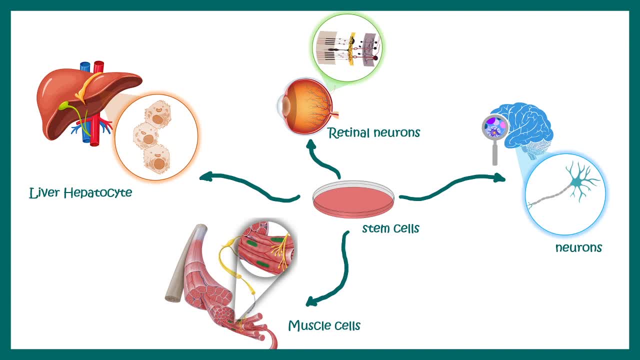 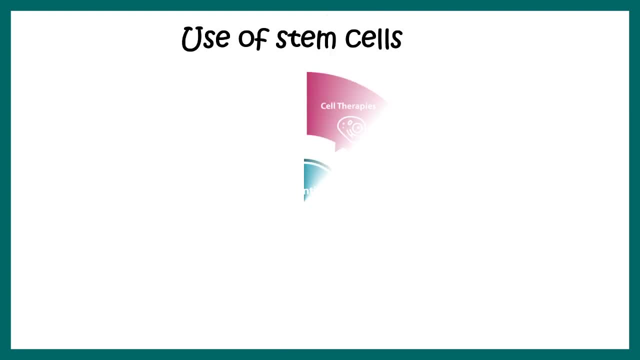 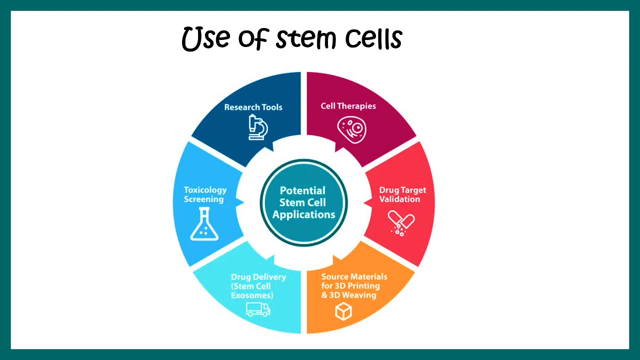 it can even give rise to muscle cells, So that is why they have versatile use in biomedical research. So let us quickly summarize the use of stem cells. They could be used for cell therapies, drug screening, source of 3D printing material, toxicology research and biomedical research tools. 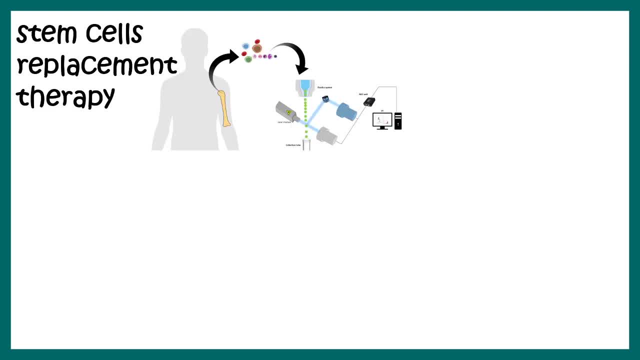 So they have wide variety of applications. So let us take a look at some of these applications. Let's say you are affected by AML, which is a blood cancer where your myeloblasts are affected. So in that situation your myeloblasts can. 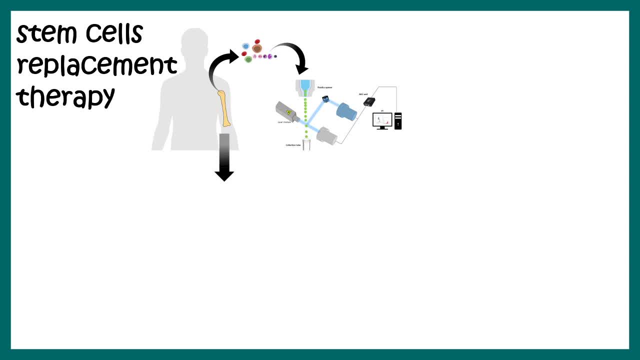 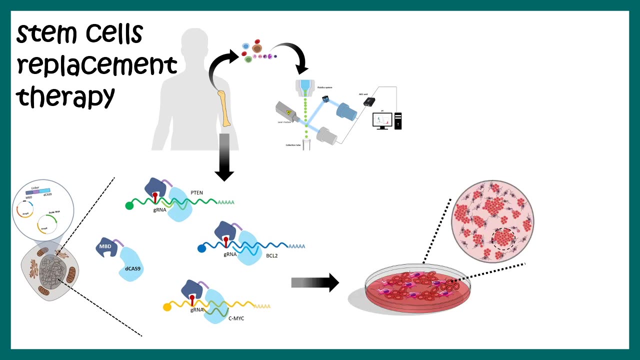 be extracted from your bone marrow, fact sorted and then, in a futuristic manner, the genetic defects in that myeloblast can be corrected using CRISPR, Cas9 technology. Once this editing is done, then these edited cells would form colony and that can be transferred back into the bone marrow. 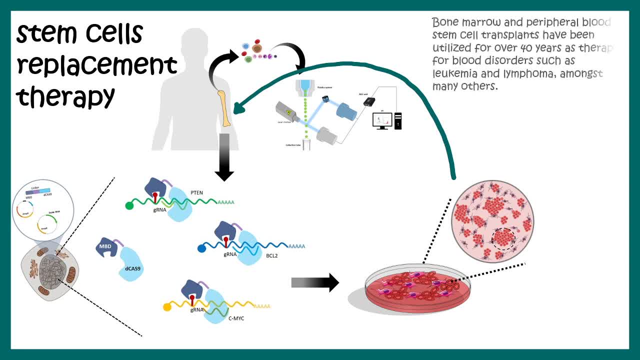 As the cells are divided from own bone marrow so they would not mount any immune response against them. So there is no chance of rejection of these cell types, and that has a huge therapeutic potential. So stem cell replacement therapy is one of the futuristic medicine approach. Let's take another example, For example. 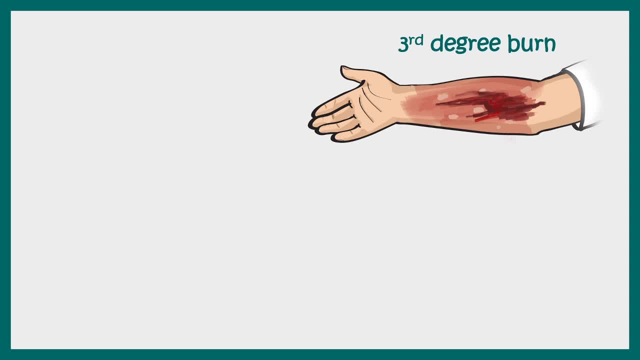 there is a third degree burn, There is a severe injury in the hand, and now the conventional treatment is taking a skin graft, preferably from this particular individual or from a person whose blood antigens are matched, and ultimately that has to be grafted onto the wound. 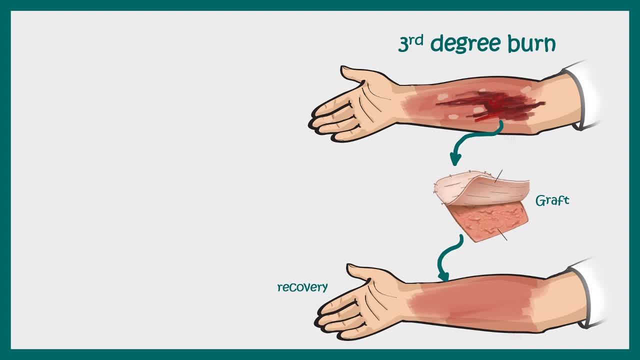 So obviously there could be a chance of wound recovery, but most of the cases it has been seen these grafts are rejected or not totally fitting in this particular situation or in this environment and there is always an inflammatory response which is creating the situation very bad. 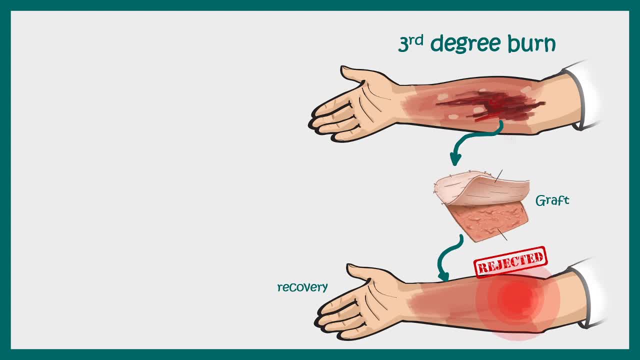 So in those situations what is possible is to take the skin cells from these individual who is undergoing this third degree burn And these skin cells can be induced to become a pluripotent stem cell. So induced pluripotent stem cells can be derived from them using these. 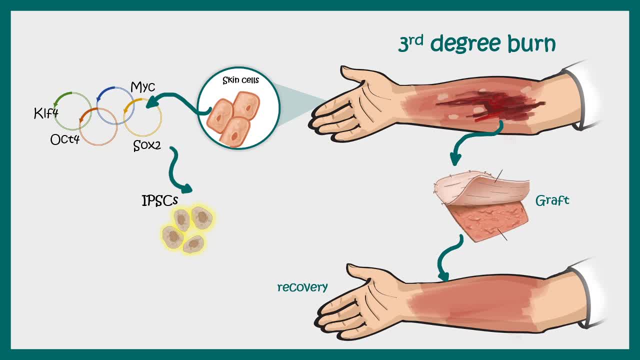 cocktail of transcription factors. Now from that induced pluripotent stem cell it is possible to culture the skin and that could be used as a graft to put it on the wound. So obviously this graft is coming from the individual who is the donor of the skin cell. so there is no chance of graft. 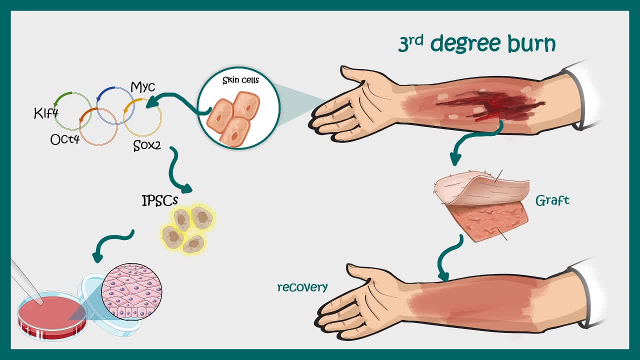 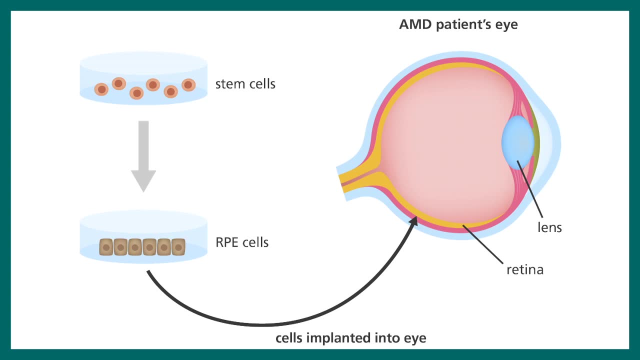 rejection, and this is another important aspect of the regenerative medicines that are futuristic Now. it would have a very low chance of graft rejection. that's the biggest advantage of this procedure. Using similar type of approach, it is possible to derive retinal cells or retinal neurons from stem cells and it could be replaced. 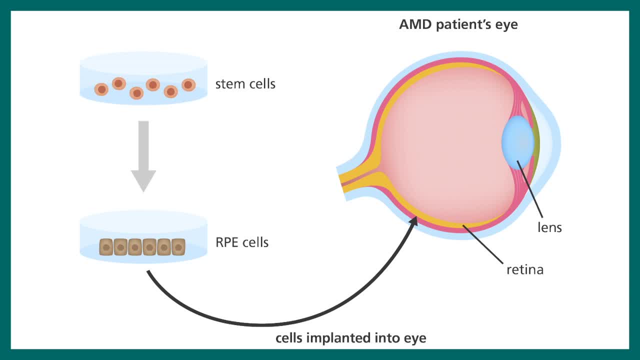 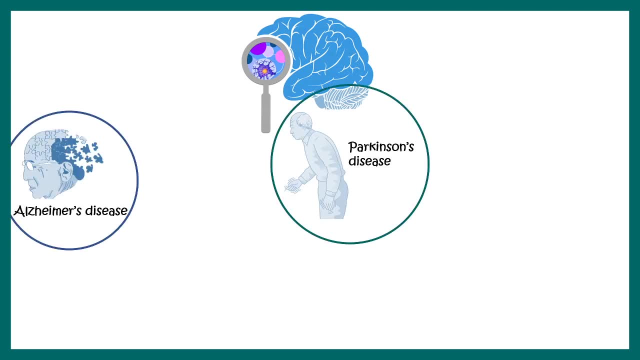 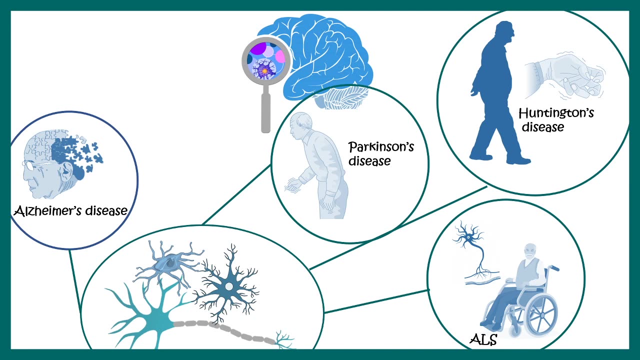 in the retina in case of severe eye disease. Let me give you an example of neurodegenerative diseases. For example, you know, Alzheimer's disease, Parkinson's disease, Huntington's, ALS. all of these things lead to change in the brain cells morphology and their viability. So many of the neurons die in these. 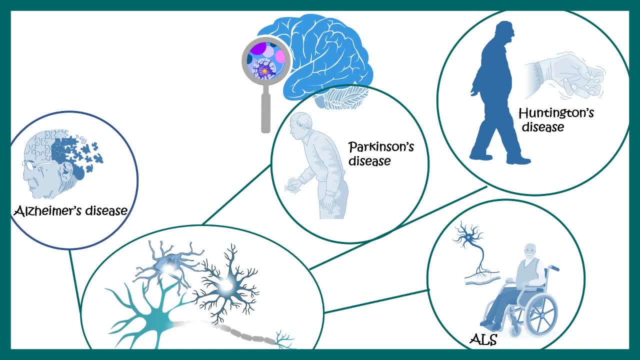 case of in these neurodegenerative diseases. So when these neurons or other brain cells, such as glia, are dying, they are going to die in the retina. So in the case of severe eye disease, it is possible, by using stem cell therapeutics to replace these neurons from. 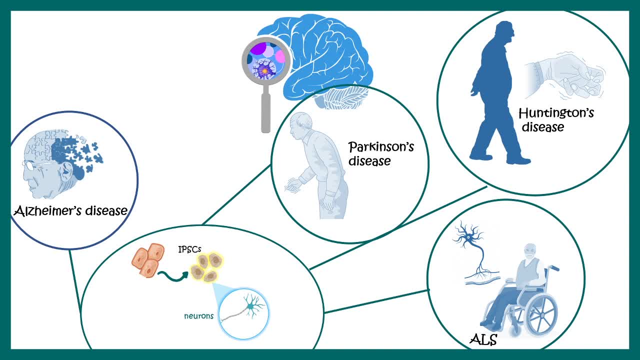 iPSC derived neurons. So obviously you can take a skin cell from these infected patients, or the patients who are suffering from Alzheimer's, let's say, and these skin cells can be converted to iPSC, which can be further differentiated into neuron, and this neuron is very much similar to the particular human from which the cell has been taken. 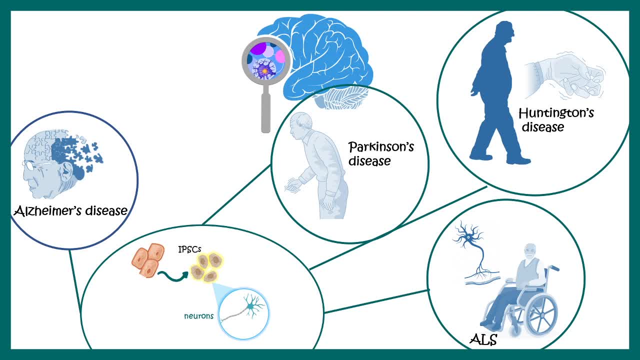 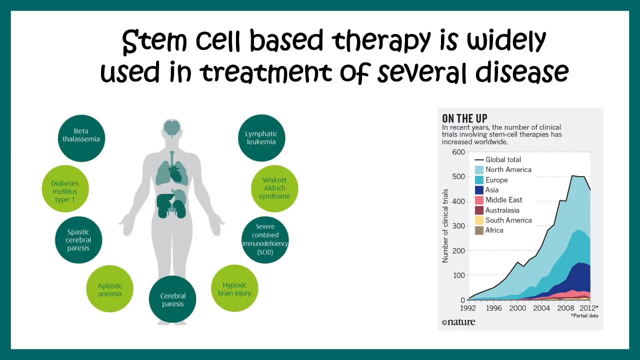 So there is no chance of rejection or inflammatory responses. So, in short, it has a huge therapeutic potential. Now stem cell based therapy is widely used for treatment of several diseases, and the usage of stem cell therapy is increasing day by day, and you can see the current medical journal. 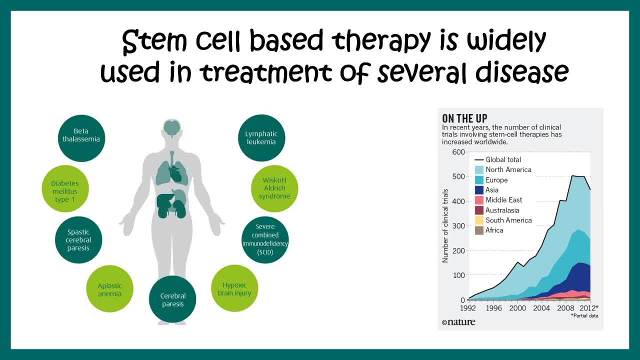 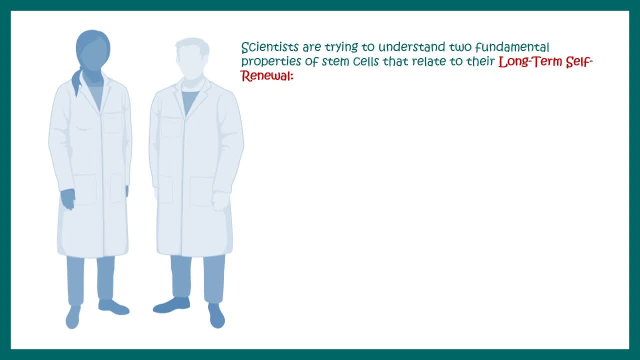 reports, and its usage is gradually increasing in North America, Europe and many third world countries as well. But scientists are really trying to understand two fundamental properties of stem cell. One is self-renewal: How these cells can really self-renew for a very long time and when it is. 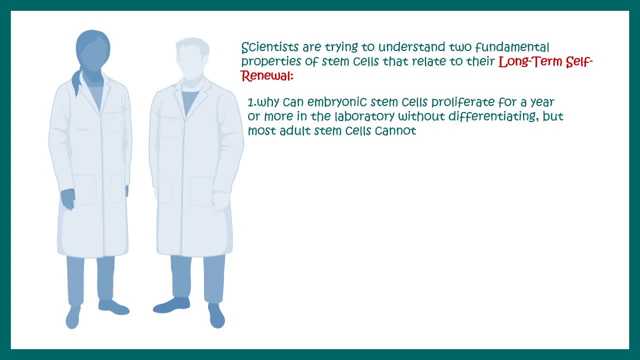 necessary, they can be differentiated into lineages. So this is the biggest question, that how this temporal aspect is maintained in by the stem cells. Second, that what are the factors in the living organism normally regulates stem cell population or stem cell renewal? or let's say, what are the 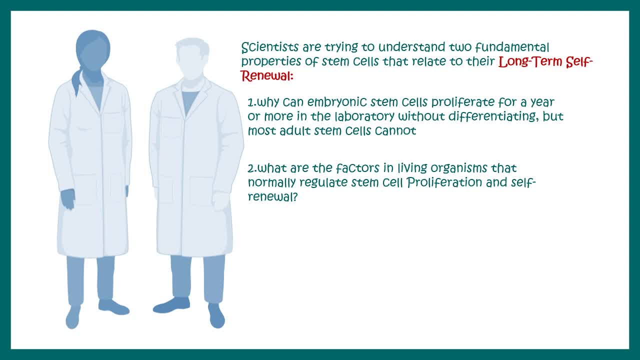 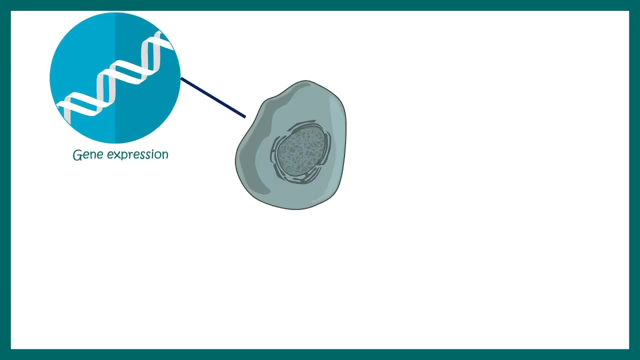 factors that kind of make the balance between differentiation versus proliferation. So these are the key questions that scientists want to ask. Also, the overarching question is: what makes stem cells different from other cells? It turns out stem cells have different pattern of gene expression compared to a normal cell. 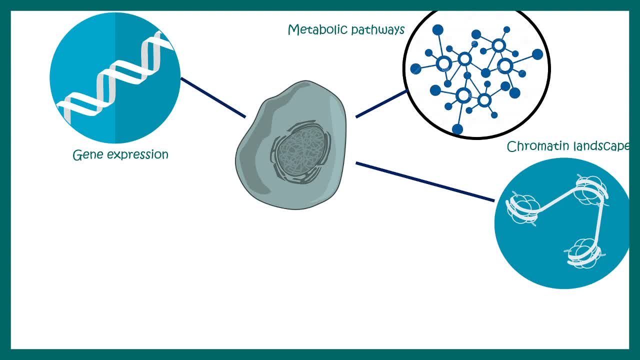 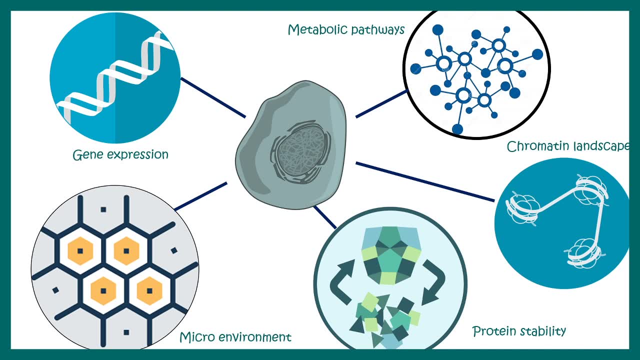 different metabolic pathways which are active, different chromatin landscape, protein stability or micro environment interaction. So all of these factors cumulatively lead to a different property of stem cells. So let us take an example: If we look at the chromatin landscape, 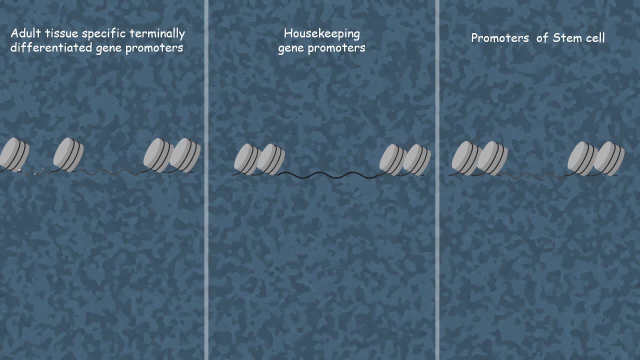 the chromatin architecture, we would see the promoters which are present in the stem cell have very different type of transcription- start site So- and which are very different from the housekeeping genes or any other genes which are regulated. Also, if we talk about the chromatin, 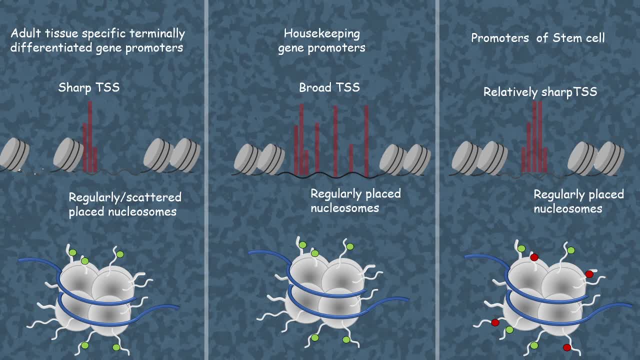 marks we would see the stem cell has equal amount of like activatory and inactivatory mark, As if the chromatin is in a poised state. it can be deactivated or silenced or it can be activated rapidly. So it's like in a charged or poised state, which is a characteristic feature of stem cell. 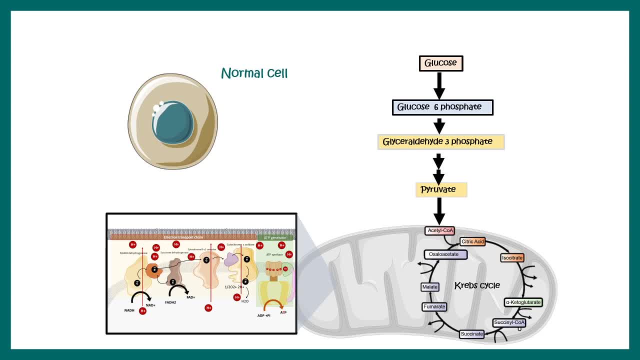 chromatin. Now, other than that, if we talk about metabolic pathway, normal cell utilize glucose and they use oxfos based method to generate ATP. and quite a lot of ATP can be generated using oxidative phosphorylation and electron transport chain, But the stem cells do not use oxfos. 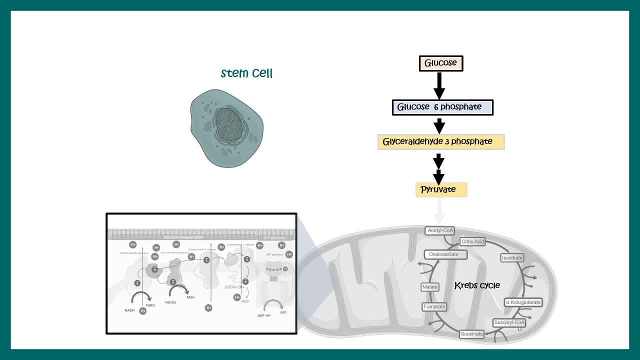 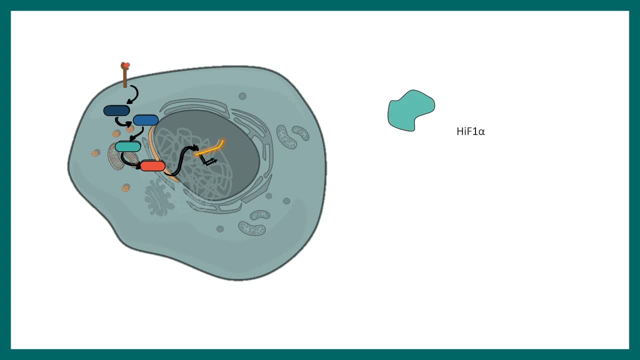 or mitochondrial electron transport chain. Instead, they use glycolysis pathways solely to generate ATP. In fact, there are several signaling pathways which are upregulating an enzyme or a particular transcription factor, which is known as HIF-1 alpha, And this transcription factor is master regulator for transcribing several genes. 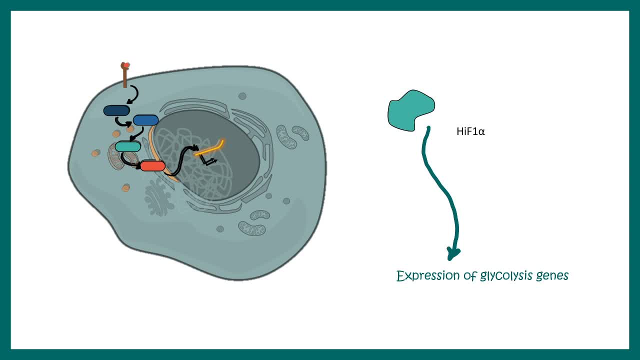 which are necessary for glycolysis. So in a molecular way, we understood how stem cells utilize glycolysis as their key fueling pathway. So obviously their metabolism is different from a normal cell which generally uses oxfos. Not only we have looked at their changes, 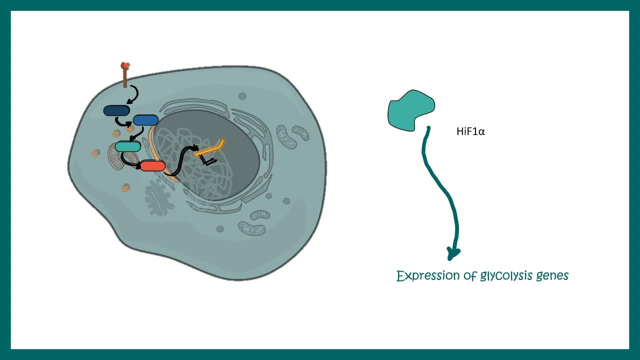 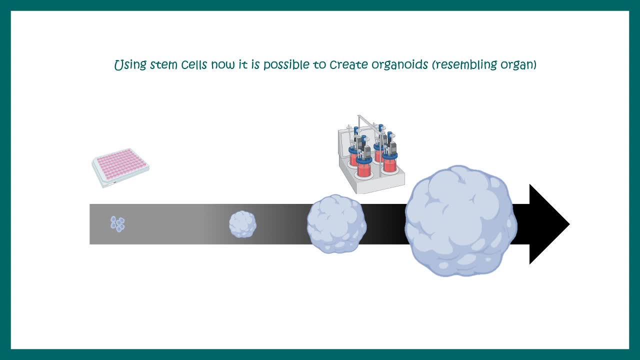 in terms of gene expression profile, but we also see how they differ from each other in terms of metabolism. Now, it is possible these days to create organoids out of stem cells. Organoids are simply meaning mini organs. So let's say, a brain organoid would resemble a brain. 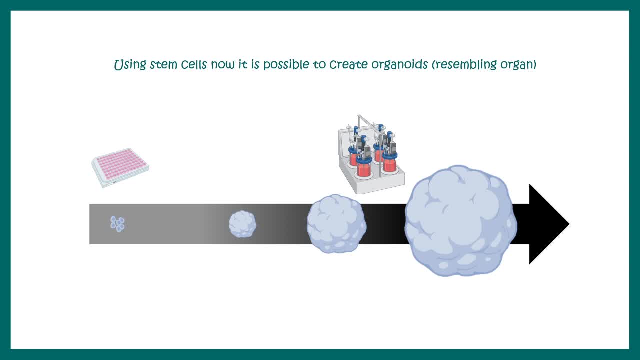 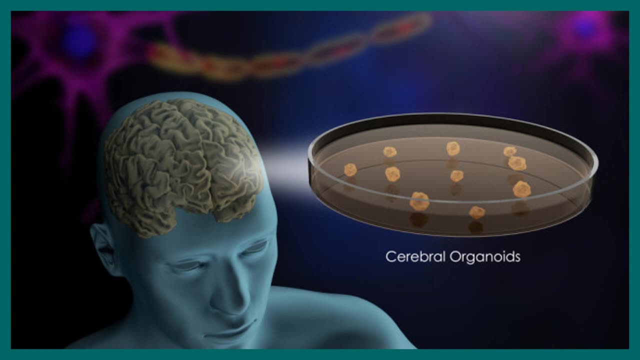 a mini aspect of a brain. Now it is possible to aggregate the stem cells and develop that aggregate in format of an organoid. Organoid would display all the necessary feature of an organ. For example, if it's a brain organoid, it would have features similar to the brain. 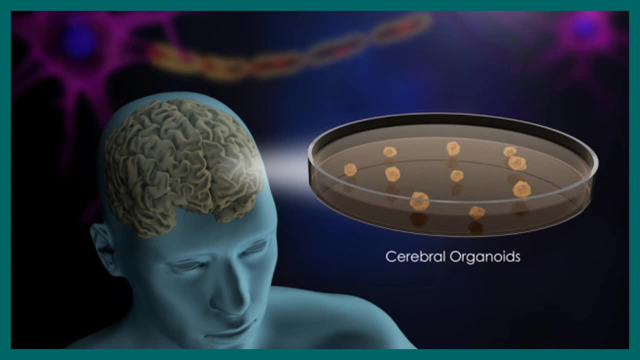 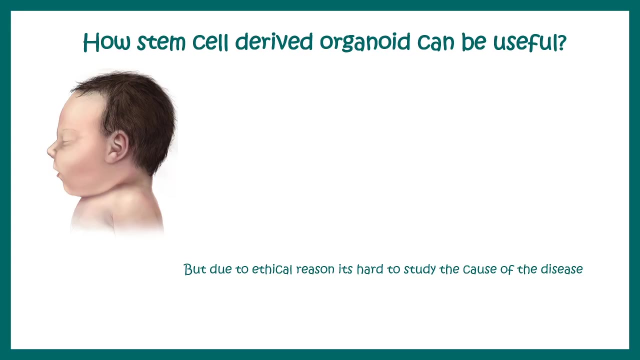 It would have similar cell types, similar properties related to the brain, And this has revolutionized the field of stem cells And it can be used for several diagnoses of diseases and many other things. For example, there is an example of a brain organoid which has been developed in. 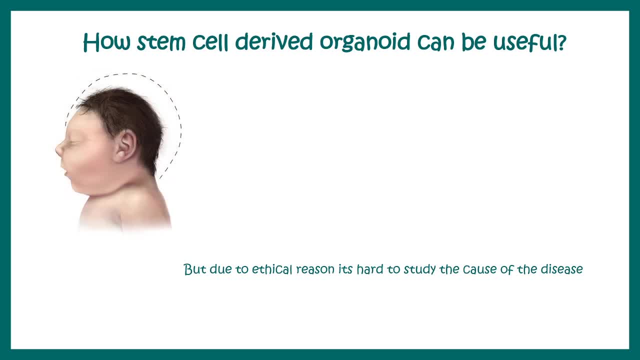 a particular facility for再 millennia. The other one is there is a disease in infants known as microcephaly, where the brain size is dramatically reduced. but due to ethical reason it's hard to study these disease and try to delineate the cause of these disease. And it is possible with 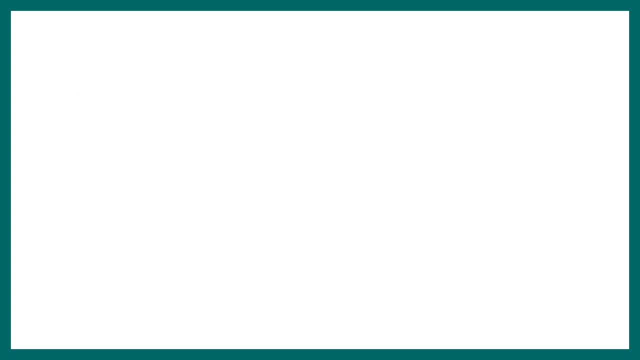 the organoid technology to look into the brain of these child. So what is done is very simple. So it is possible or ethical to take skin cells from these babies to induce pluripotent stem cells from which these cerebral organoids can be derived, and by analyzing these cerebral organoid from a cellular and molecular 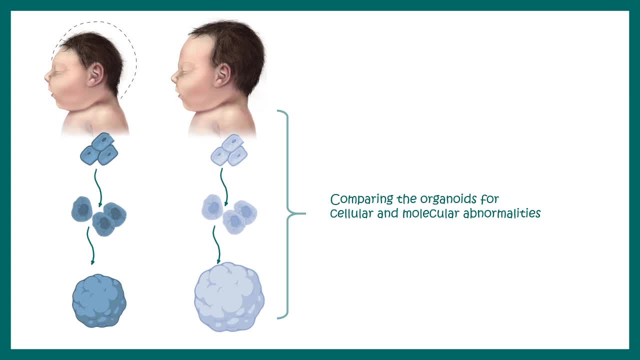 point of view we can understand what really goes wrong in these kind of diseases. these kind of diseases was totally impossible to study because the baby would be inside mother's womb and it is totally unethical to manipulate anything inside. so but we can generally take their skin cells and we can you. 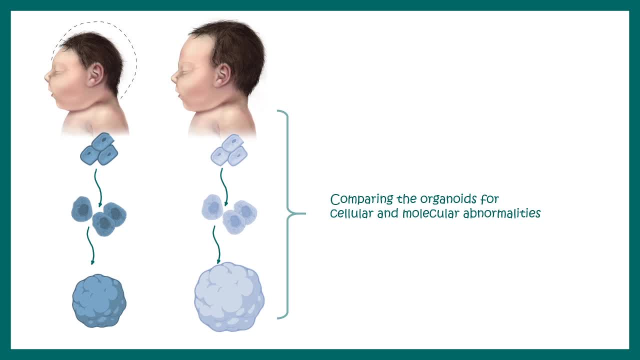 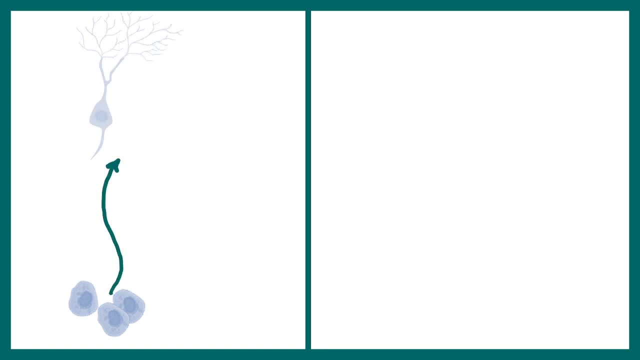 make organoids to study what is going wrong in the brain, and this has been done already. so, and it has been noted that generally stem cells give rise to neurons, but they do so by really proliferating at a very high rate, so first they increase their number and then they get differentiated into the 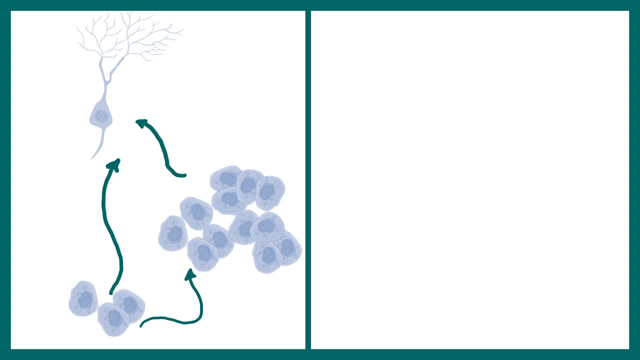 neuron. so this is happening in the normal babies, but in case of these mice they are not differentiated from the normal babies. so they are not differentiated from the normal babies. so this is happening in the normal babies, but in case of these mice microcephaly that we have talked about, scientist looked at the organoids. 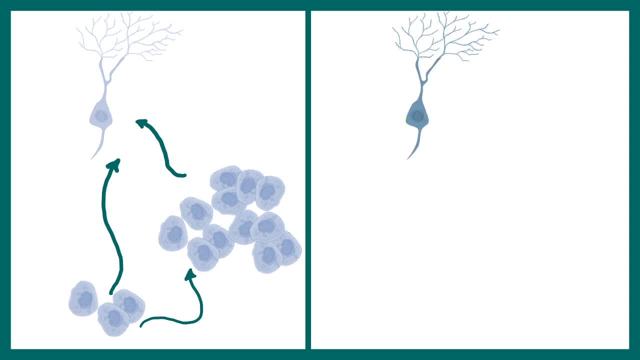 which are derived from these microcephaly babies. they get differentiated very quickly instead of amplifying their pool. so their stem cell pool is very quickly exhausted and after point of time they cannot produce too much of neurons. so they start producing neurons very early, but they run out of energy and cannot. 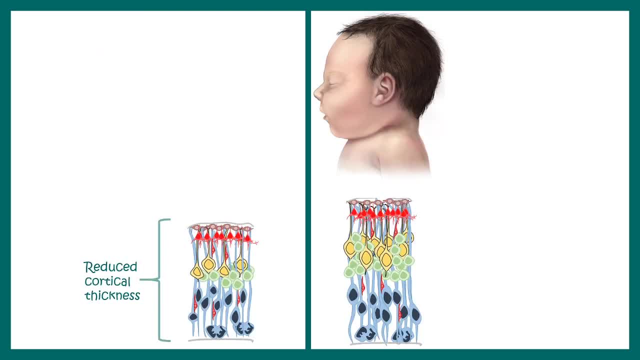 produce it further. so as a result, there is a shrunken cortex outstanding, higher cortex of these babies, which is leading to this kind of morphology shown in this diagram. So these kind of neurodegenerative diseases or neurodevelopmental diseases- their fundamental aspects, could be studied using stem cell therapy. Now let's talk about Alzheimer's disease. 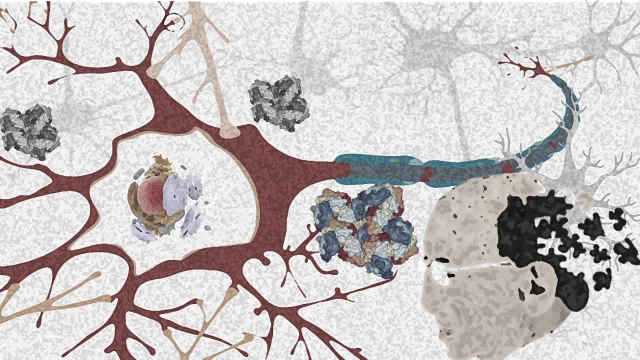 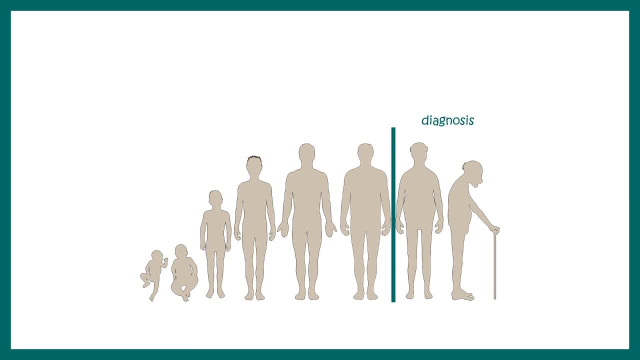 Alzheimer's disease is a neurodegenerative disease which affects the older population. Now you know these diagnosis that tells you that you have Alzheimer's happens pretty at pretty old age, and it's really impossible to diagnose Alzheimer's at very early age, before the symptoms are visible. 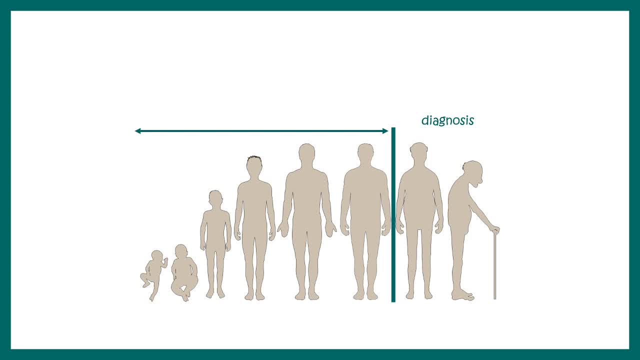 even if you have a family background of Alzheimer's, nobody really taste it because it could be dangerous. for tasting these things right, Imagine things would be very easy with these organoid stem cell derived organoid technology, because you just need a skin cell and you can convert this skin cells into a organoid cell. and these organoid cells can't. 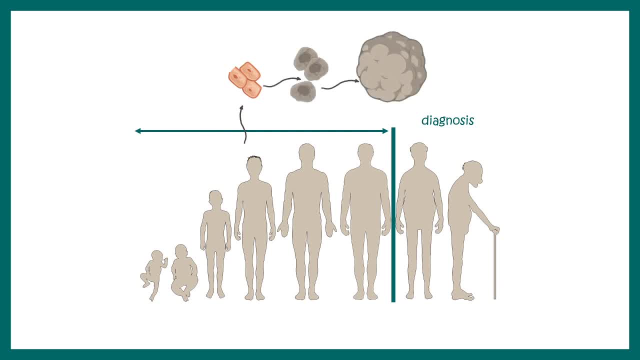 change skin color. they can't change the color of your skin, So you can't change your skin color cell into induced pluripotent stem cell and thereby making an organoid out of them. this organoid would resemble the brain of these potential alzheimer's infected person. so by 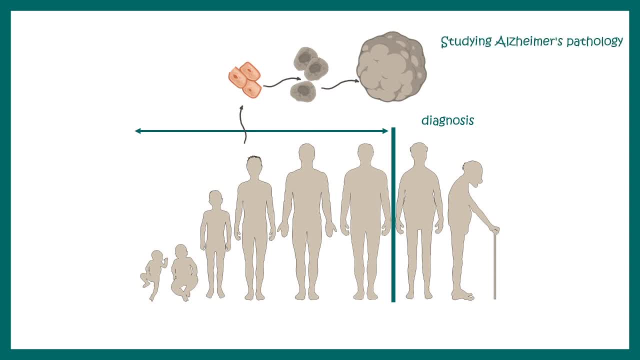 looking at the organoid. it is possible to look at what has gone wrong in these brain derived organoids, as if we are getting a picture of the pre-clinical stage or the pre-symptomatic stage. this would give them more time. it would also be useful for a better management of these disease. 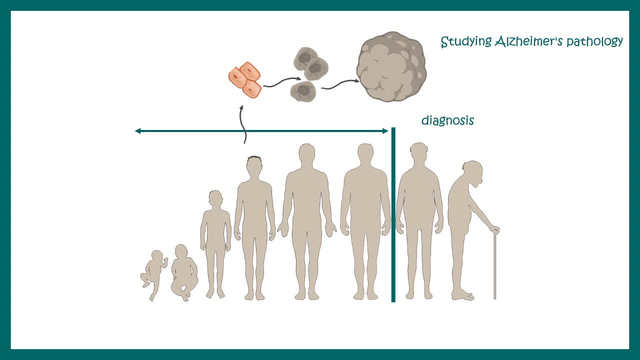 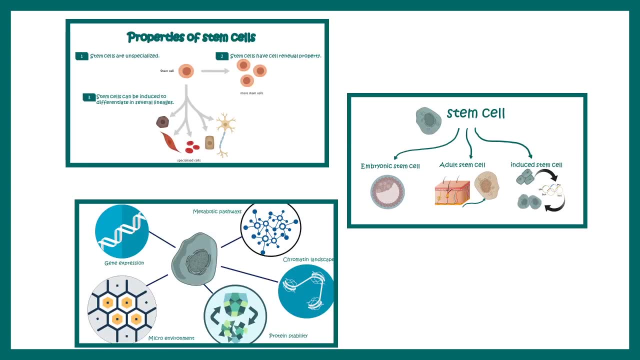 and it's fantastic, but all of these sci-fi techniques are on their way. there are quite a lot of advancement going on in this field every single day. so in this video, what we learned is the properties of the stem cells. we learned about the stem cells classification. we looked at embryonic 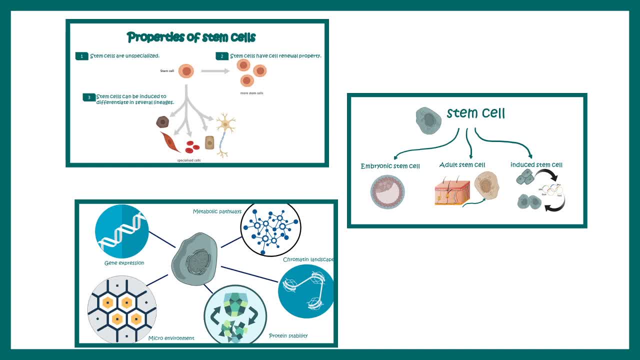 stem cells, adult stem cells, etc. and lastly, we looked at the metabolism of the stem cells, or the aspect of stem cells which make them really different from other cell types. so that's pretty much it. if you like this video, give it a big thumbs up. don't forget to like, share and subscribe, and do. 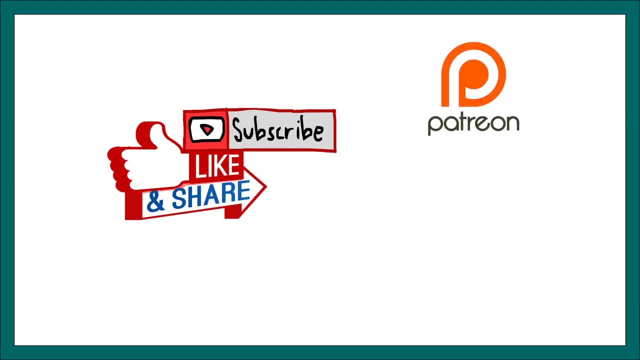 subscribe to my patreon page. you can also support me by paying me five dollar in patreon. your support would be valuable for me. and if you like to join my course in unacademy, please use my code epitane to get a 10 discount. unacademy is india's biggest online learning platform. with that you can do. 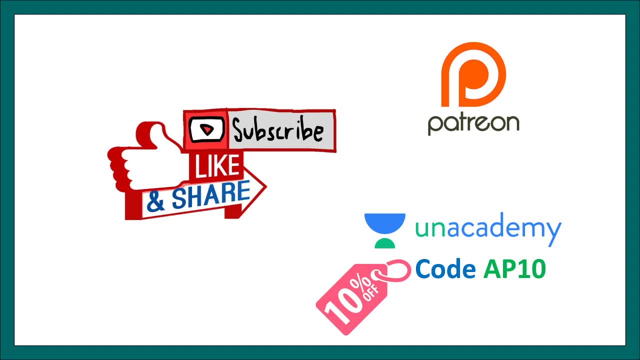 smart learning. you can learn from wherever you want, whenever you want, so please subscribe to my channel. thank you, guys.